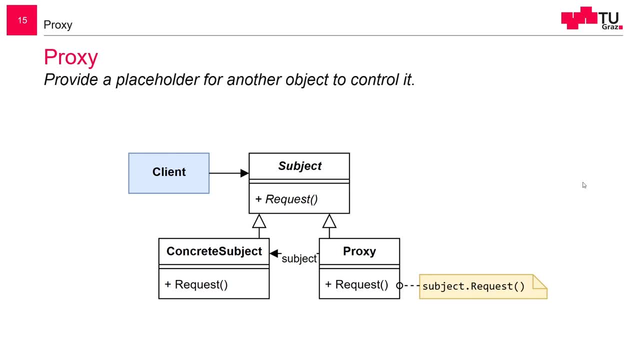 The proxy pattern. The idea behind proxy is that we want to get a placeholder for another object in order to control it. This placeholder should be transparent, so it should have the same interface as the original object. As you see in the diagram, a client calls the method of some subject. 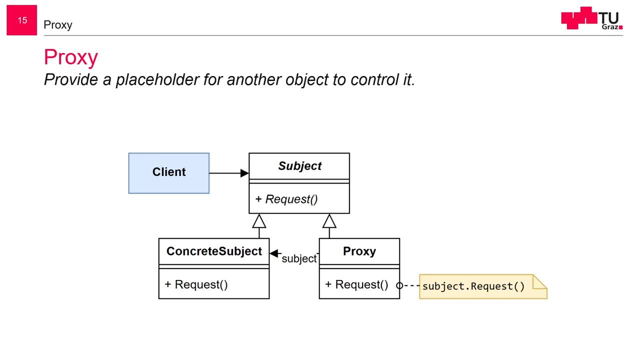 Here the subject is already an interface. We want to have this request method In order to do that. we could either create a concrete subject, a subject which implements this subject interface, or we could implement a proxy which uses this concrete subject under the hood. 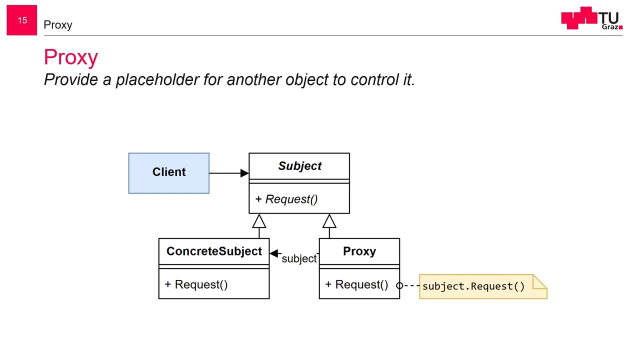 Basically this is again the same idea as the object adapter: that we use another object under the hood, but in this case the interface stays the same. The adapter changes the interface. the proxy leaves the interface the same. The context is that we have some objects. 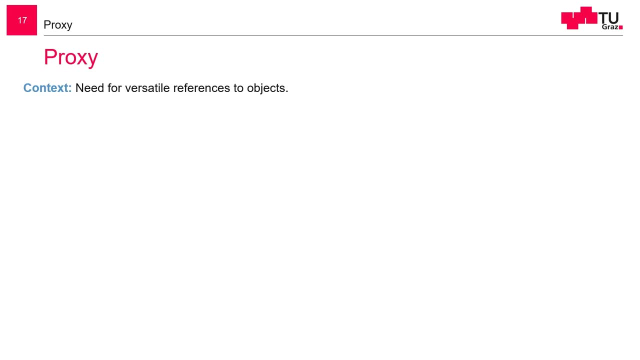 and these objects maybe sometimes need long to load or should have additional things checked before we access them. So we need some versatile references to these objects, And the problem is now: how can we handle such objects which are not directly accessible? And, of course, the answer is to use a proxy. 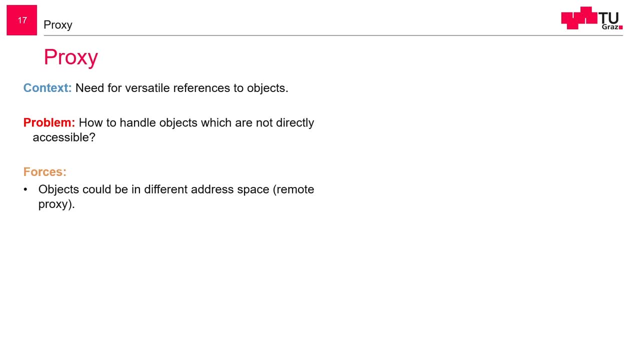 For example, objects could be in different address spaces. For this a remote proxy or a communication proxy would be interesting- And this proxy has the task of dealing with this. serialization and the communication parts in between, Or the object takes very long to create. 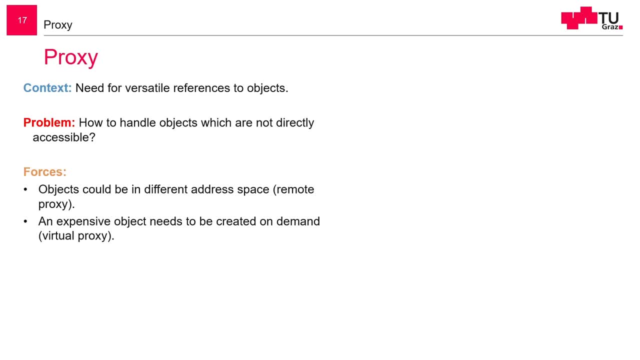 For this we could use this lazy loading proxy, So a virtual proxy which represents the object, the original object, but just as a handle, And if we want to access the properties of the object, then we create the object actually, And this could then take some time. 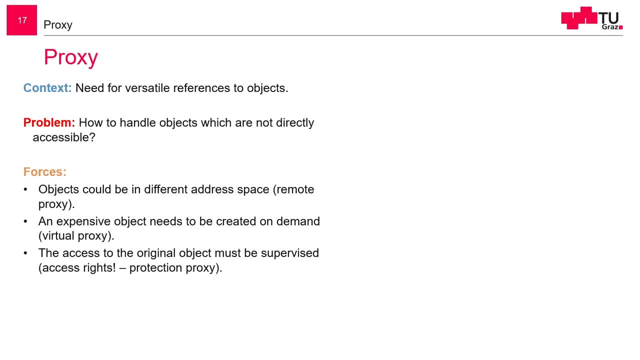 Or we want to check the access rights of objects. Can every object be accessed by all threads in our application? Or maybe we want to restrict our access rights? Also, proxies can be used as smart references, For example smart pointers or unique pointers. 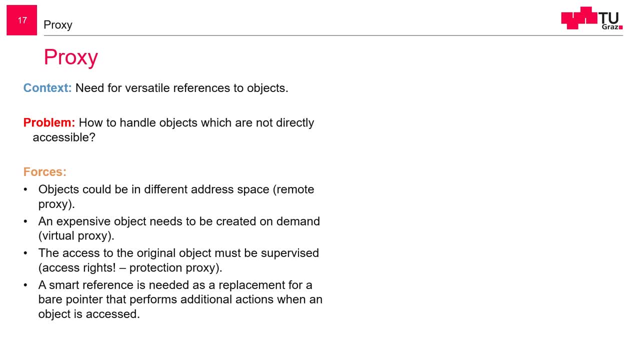 So they should behave like pointers but have some additional stuff and some additional semantics behind them. So the solution is to give a reference, a placeholder class to the client which has the same interface but accesses the real object underneath, And of course it should reroute all the calls to the real object. 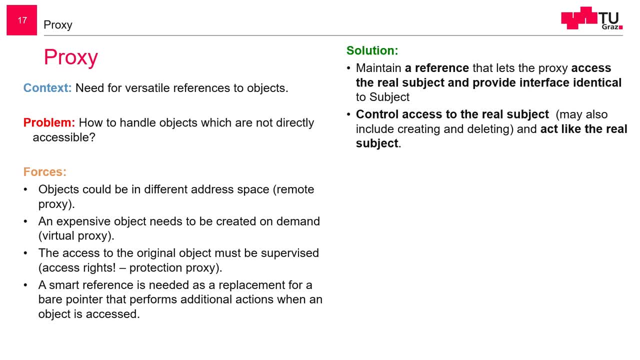 It should act like the real object or subject. It's always called subject in this pattern, So it's completely transparent to the user that the object isn't, for example, at the own machine, but at another machine, And that's the idea of the proxy. 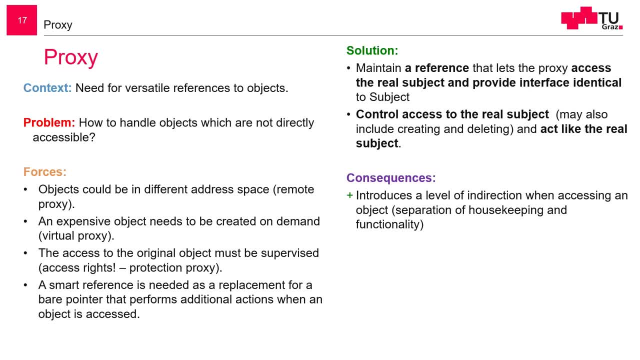 So the consequences is it introduces another level of indirection. So this can actually be a drawback also, For example performance-wise. we have another call, another layer in between of the direct object. But for the proxy we can use this, for example: 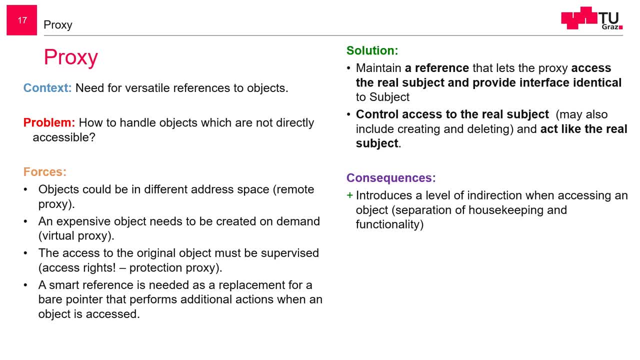 for housekeeping and for storing references and only loading these resources which we really need. So yeah, A remote proxy can decouple client and server, So it can be that we communicate via the network without even knowing it. So remote procedure calls. 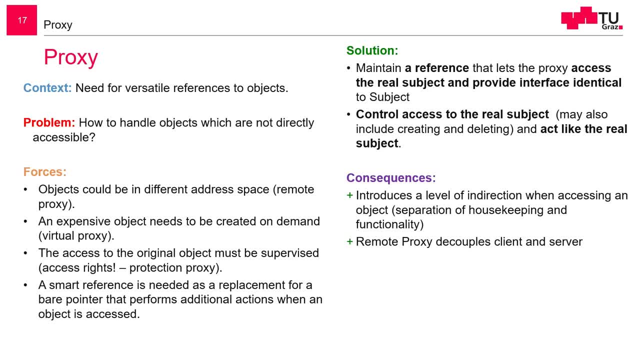 a proxy for remote procedure calls would be perfect for this. Then a virtual proxy can perform optimizations by loading objects later on, only when we need it. Caching proxy and caching and pooling is a design pattern which we will handle in later lectures, But the caching proxy could.